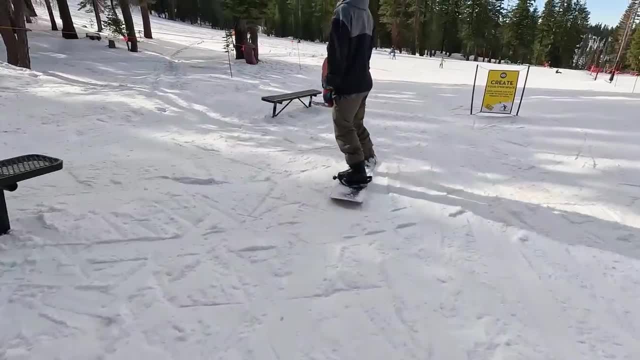 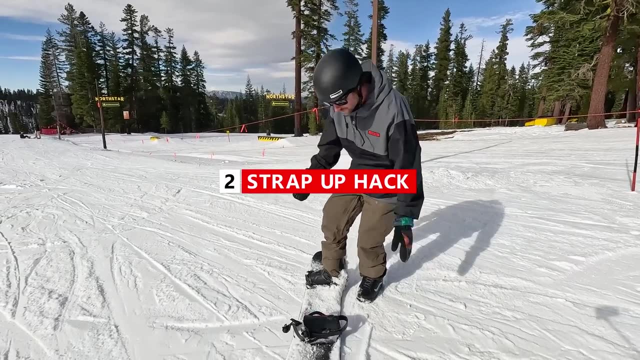 snowboard onto your free foot. We've got four more to go. The second hack will help you for putting on your snowboard. So it's very typical, especially when you're just starting to have to sit down and strap up. but by doing it this way, eventually 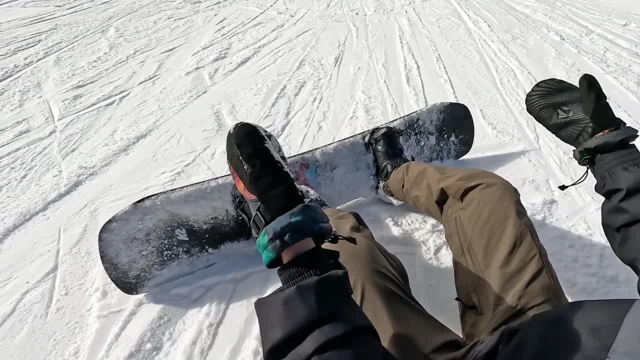 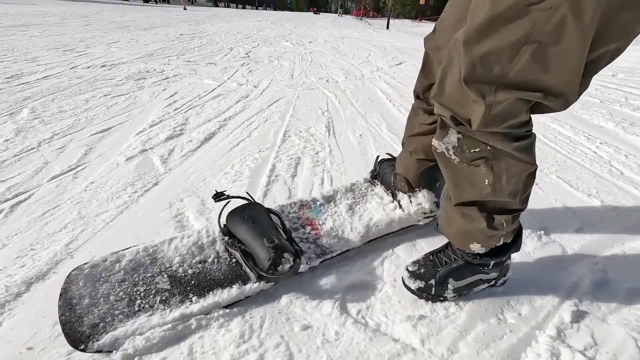 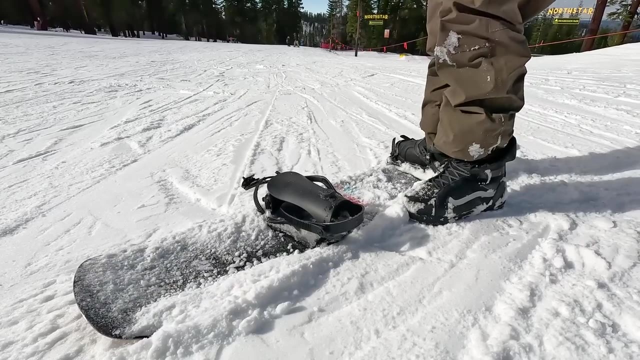 your butt is going to get wet and cold, and then you have to stand up out of the snow. So instead of having to go through that whole process, you can dig yourself a shelf. So take your heel edge, start digging it into the snow and do it until you have like a nice little platform. 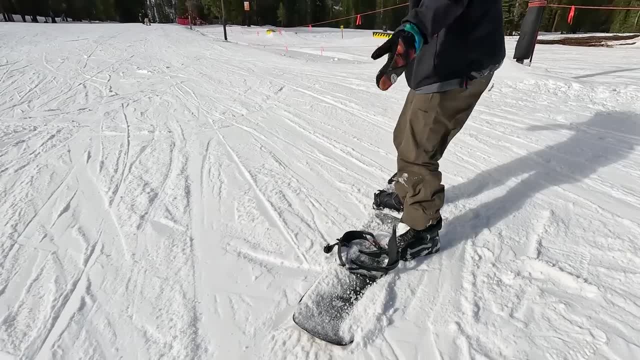 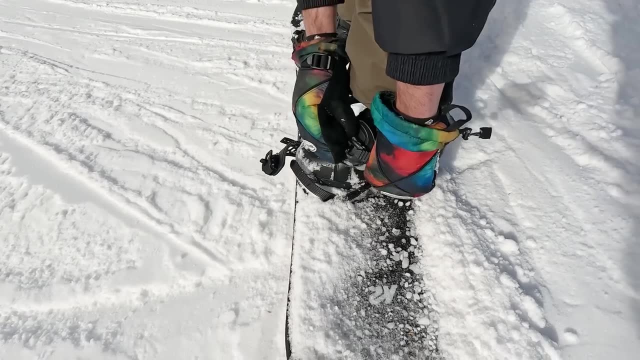 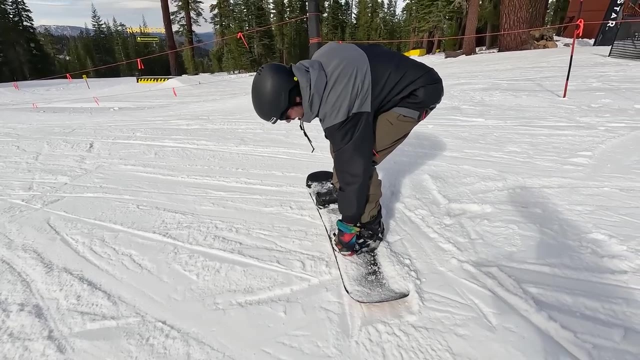 where you can stand up and put your binding on. So by doing it this way, it's going to prevent you from having to sit down With this shelf. I'm very comfortably just standing here and easily strapping up my bindings without having to sit in the snow and get all wet. 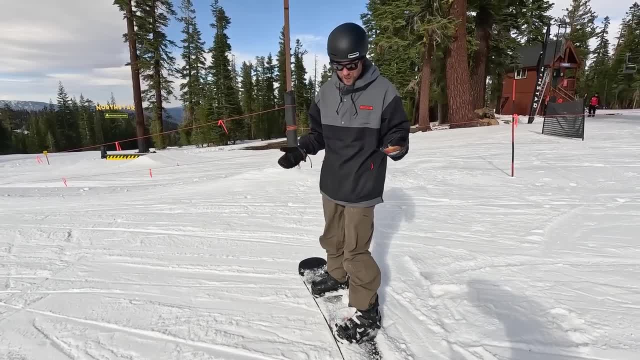 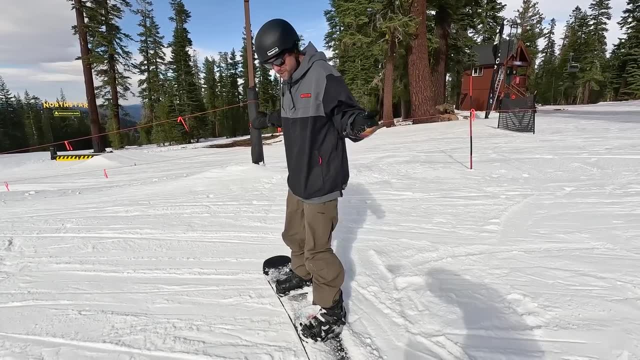 If you can do it this way, you're going to stay much more drier and warm through the day. Also, you don't have to go through the struggles of sitting down and getting up out of the snow every single time. Now, from this position, I can just start to ride and start my run. 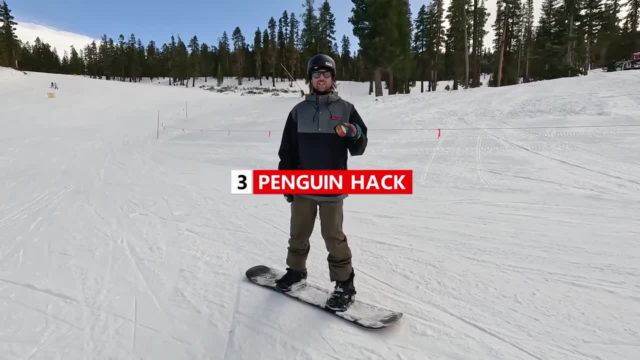 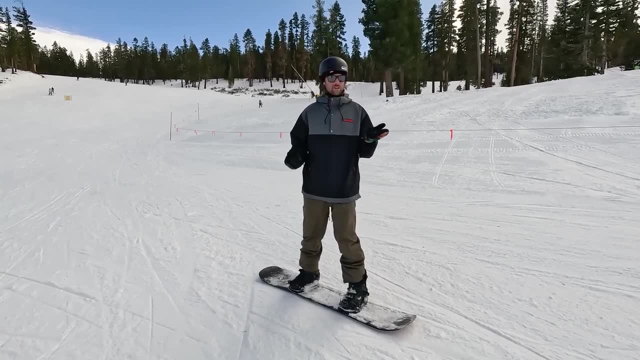 The third hack- and this one really specifically applies to snowboarders- is when you get stuck in a flat area and as snowboarders we don't have like poles or anything to push us across, So our only option is to really unstrap, walk across where we want to. 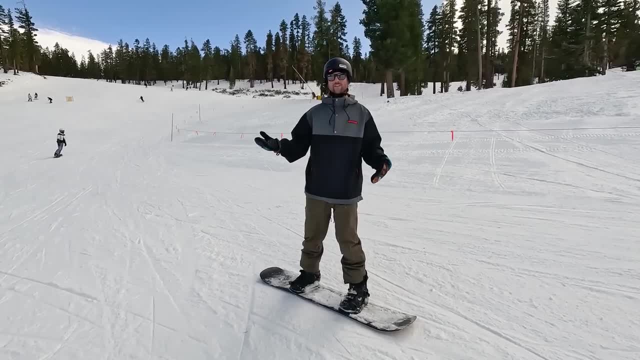 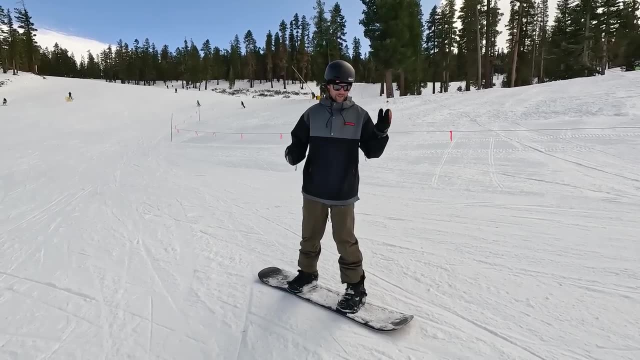 to and then do the whole process of strapping up again and then going down the run. But there's actually a hack that you can do to skip all that and get across the flat areas, and the hack is to do the penguin walk. So the penguin walk is pretty simple. it may take a bit of practice but it's. 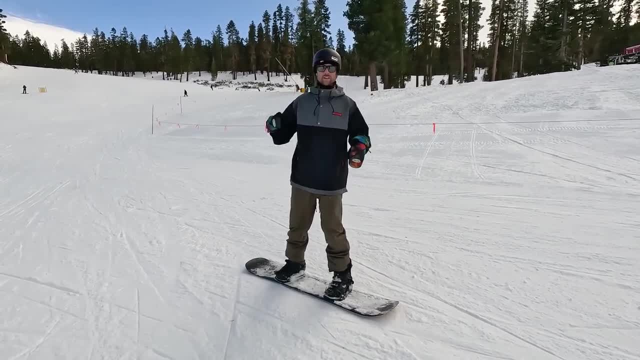 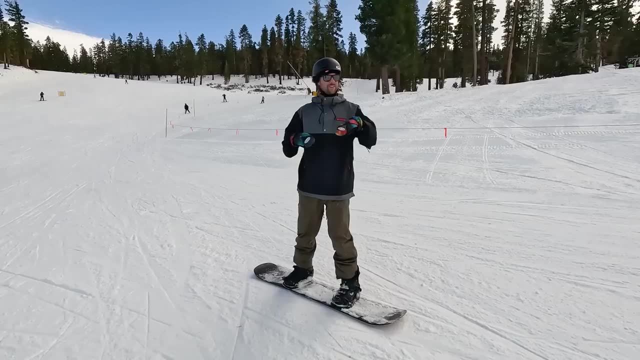 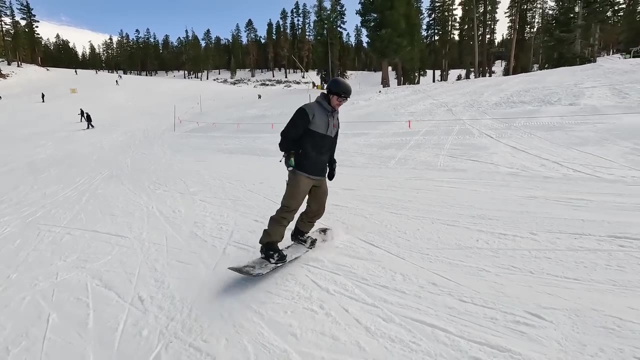 getting your toe edge in the snow and then alternating between your nose and tail and just like walking and pushing yourself across the flat area. So this is an amazing hack: if you ever get stuck in a flat area, you can just quickly get out of it. Here we go, So nose, tail and just keep. 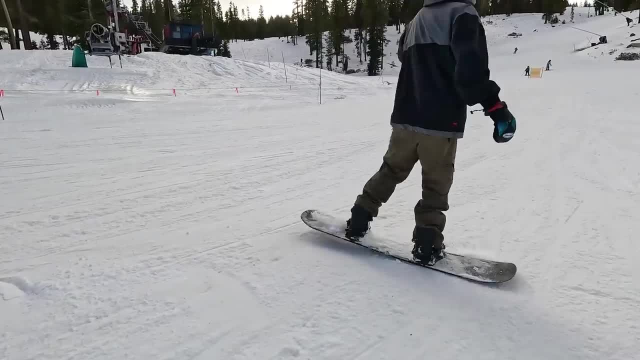 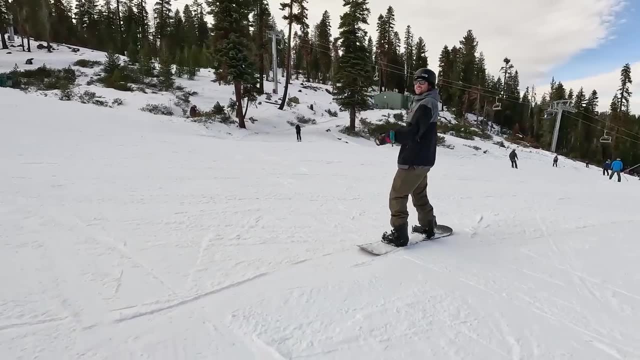 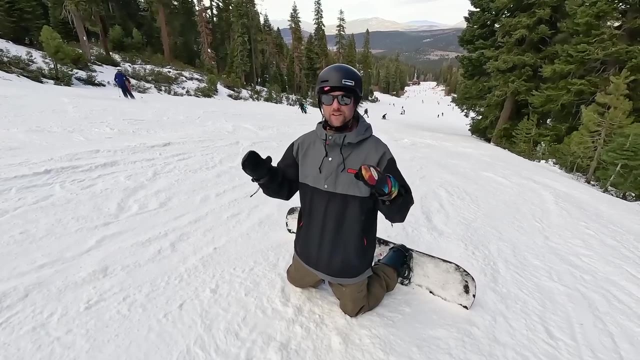 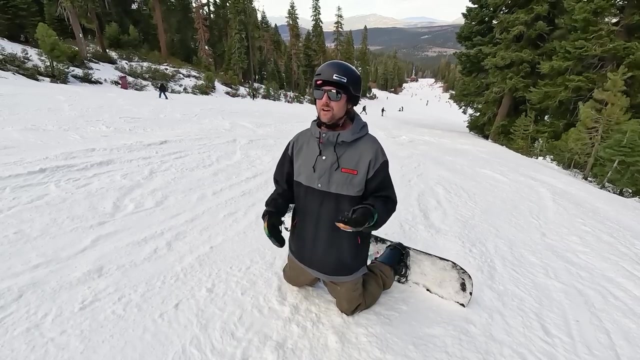 pushing myself across with my toe edge, So alternating between my nose and tail, pushing myself across until I'm free. The fourth hack is if you ever need to stop the run. it's super common to either go down on your knees or sit on the side, but a much. 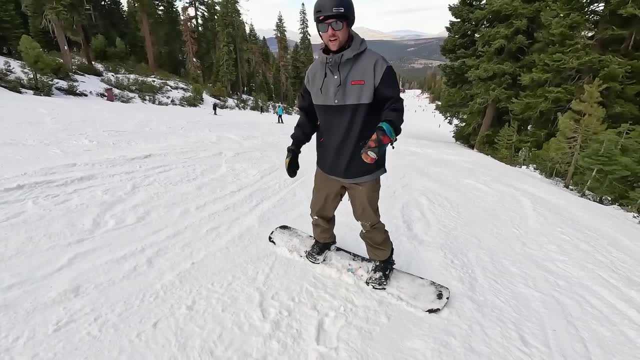 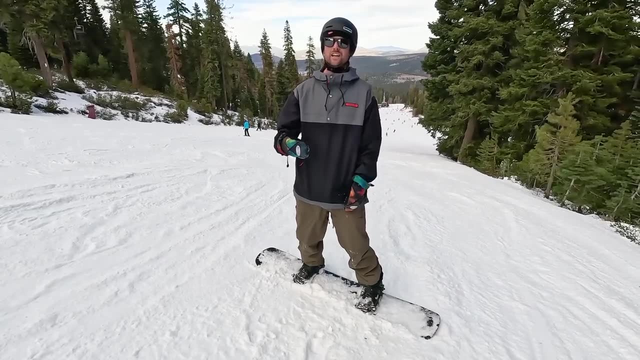 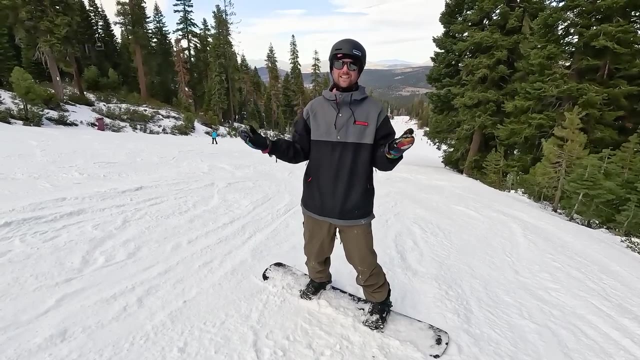 better way to do it is to just dig yourself a shelf, but this time on your toes. So by digging yourself on your toes you can stay standing on the side. It's much better safety-wise, because now you can see everything above you and also if somebody's coming down, they can see you better. 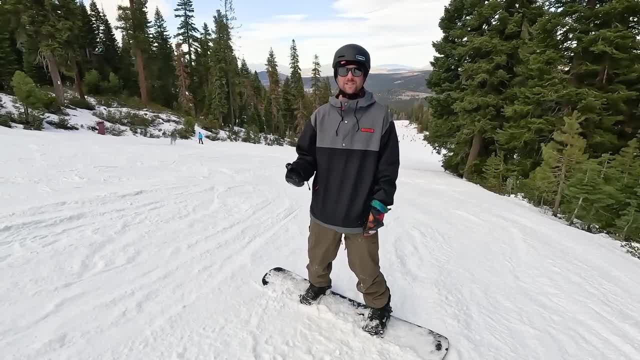 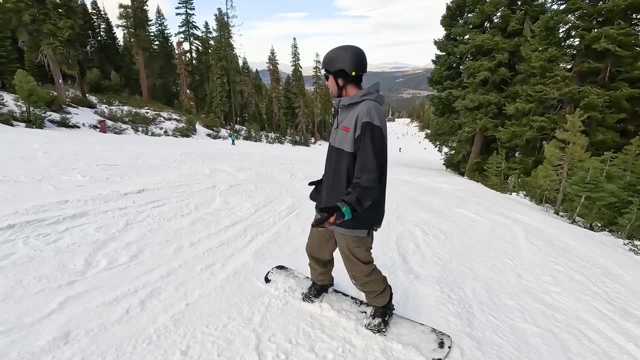 and if, for some reason, you need to get out of the way, it's going to be much easier from standing, So, safety-wise, this is better. It's also going to keep you drier being up out of the snow, and I think it's just a better way to rest. 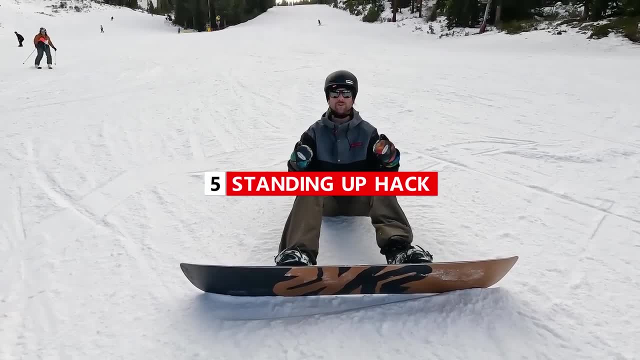 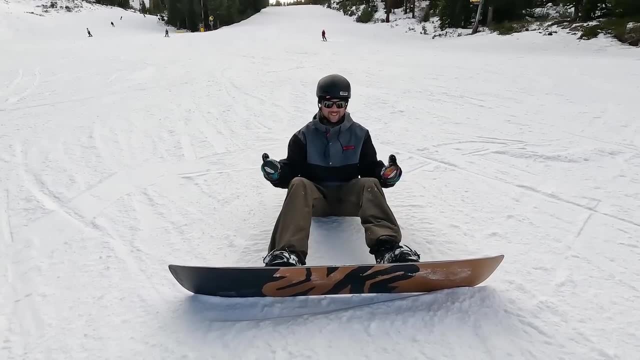 So the final hack, and this one is for standing up If you do find yourself sitting. so if you're a beginner snowboarder practicing your heel sliding or just in general, you find yourself sitting in the snow. if you don't have the best flexibility, it can be really tough to stand up. 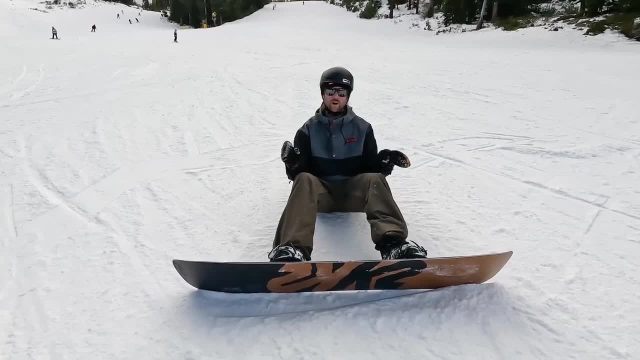 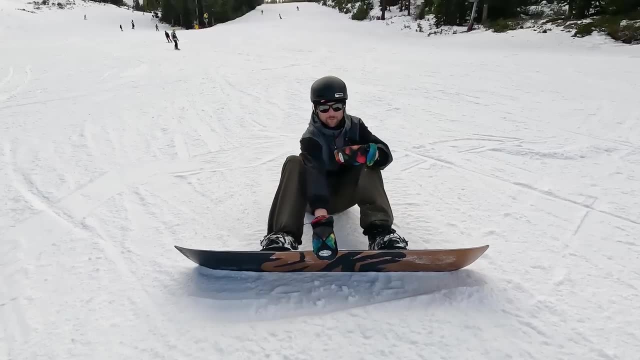 from your heels. There's two ways to do this. One is to actually take your front hand and grab the toe edge of your snowboard so, like now, you have something to pull on to bring your board closer to you as you push up with your back hand. 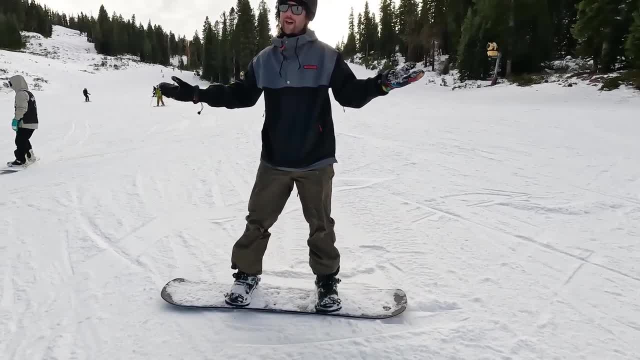 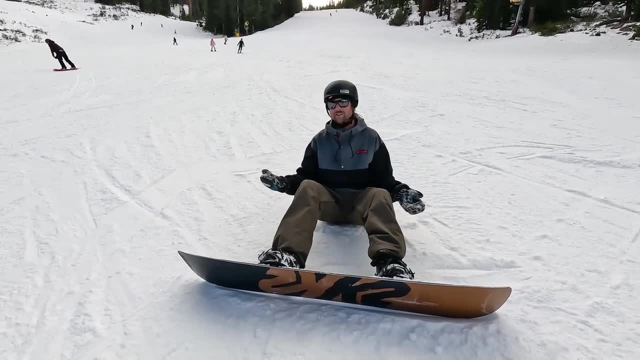 So I'm pushing and pulling and then you can stand up that way. The other way to do it, which is probably much easier, is to just roll over onto your toes, and instead of struggling to roll over, you can just grab behind your knee with one hand. 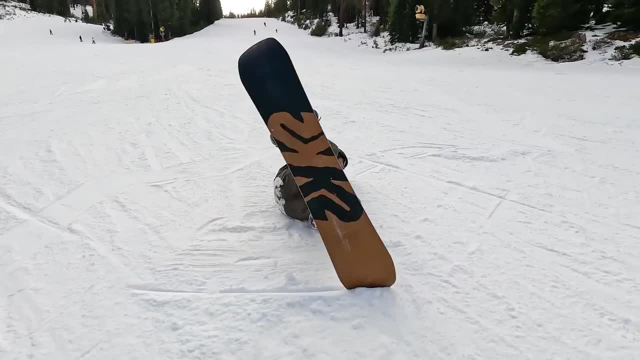 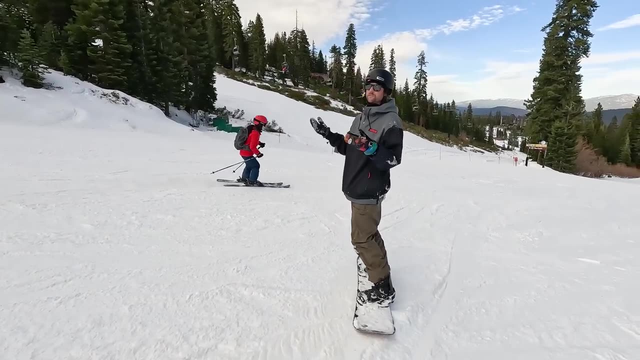 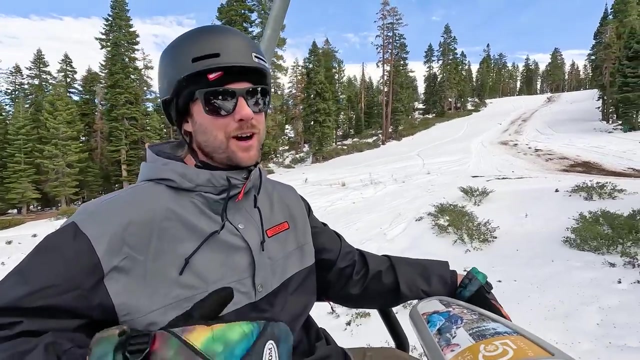 and then, as you roll over, just pull this knee And so that's like two easy ways that can help you stand up from sitting. Amazing guys. so I hope those five hacks will help you on your day of snowboarding. Just remember, when you're sitting on the chair, rest your snowboard on your foot When you get 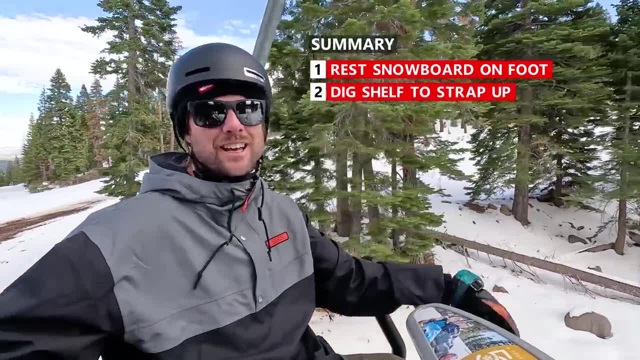 off the chair and, strapping up, dig that shelf so you don't have to sit down. If you do get stuck, try the penguin walk that I just showed you. If you do get stuck, try the penguin walk that I just showed you.